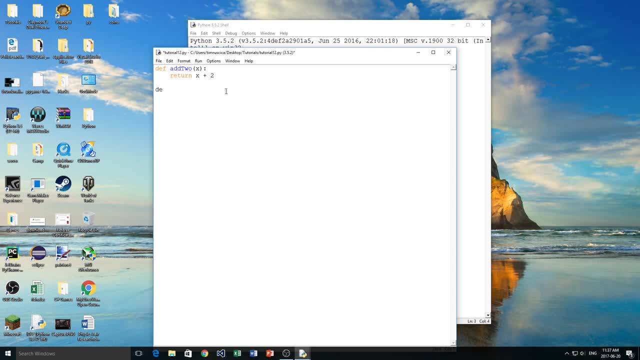 So if we wanted to make our own function, what we would type is we'd type def- this stands for definition- and then the function. So maybe in this case I want to do another math-related function, so I'll do subtract2, and oops 2 as a word, and then I'm going to put two brackets. 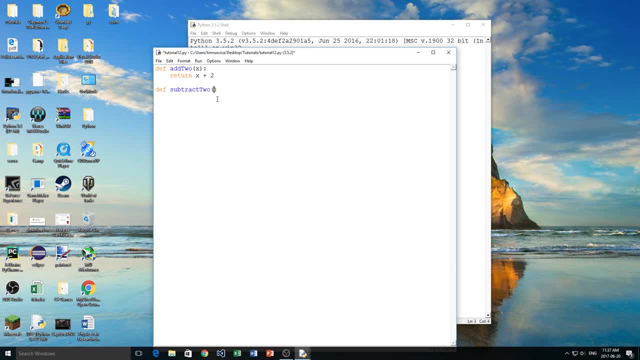 and inside of the brackets we're going to put something that's called a parameter, So in this case I can name it anything I want. I'm going to put number in here and then I'm going to do a colon: click enter. it should tab me in one space. 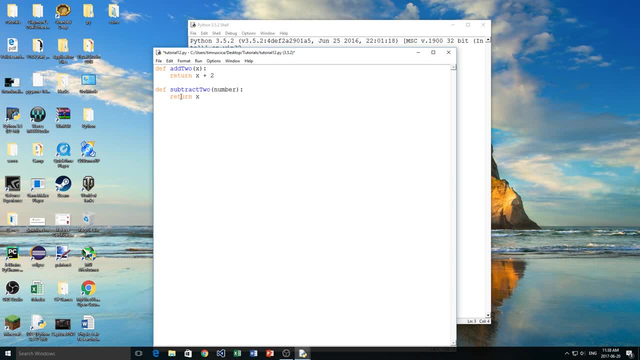 and I'm simply going to return x, or sorry number, Minus 2.. Now I'll talk about what all this really does a little bit later, but I just want to give some examples. So now, if we want to call our function, or we want to actually use these functions, we have to do something. 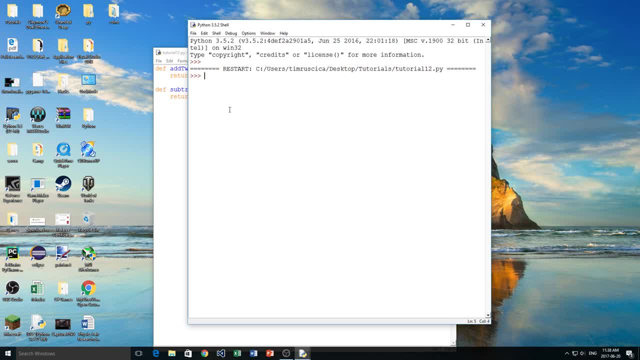 We can't just leave it like this. I'll show you: if I run this right now, nothing's going to happen. What we actually have to do is we have to do a call statement. So what I can do is I can do addTo, and then in here we have a parameter x. 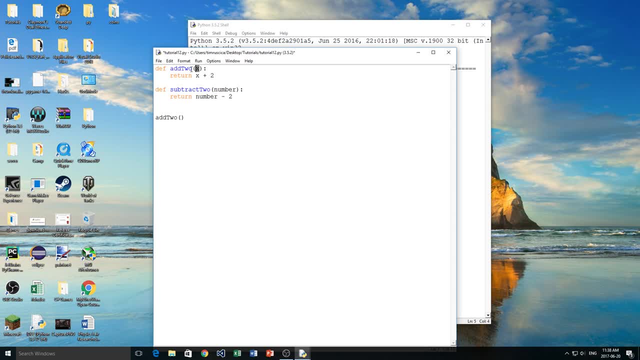 But what's actually going to happen is I have to give addTo a number, because we're going to addTo to that number and it's going to be returned. So let's say 7.. Now you'll see what's going to happen here. I'll run it quickly and nothing prints out to the screen. 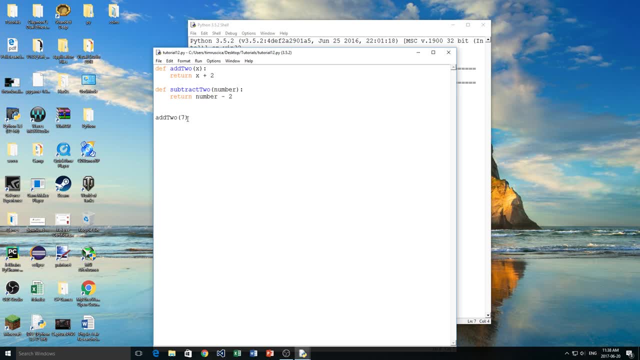 That's simply because we haven't printed anything. What actually happens is in this addTo call statement we have it sets x equal to 7, so it comes up here and it says: okay, we're going to add 2 to 7.. 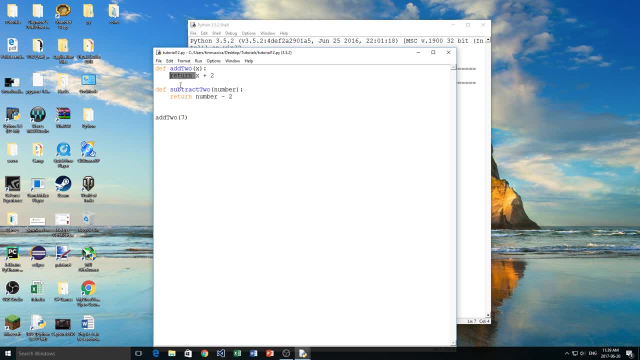 So we have x here, we add 2, and then we're going to return that back down here. So pretty much we call this function and it returns it right here. Now I have to set this equal to a variable or simply print it out to the screen. 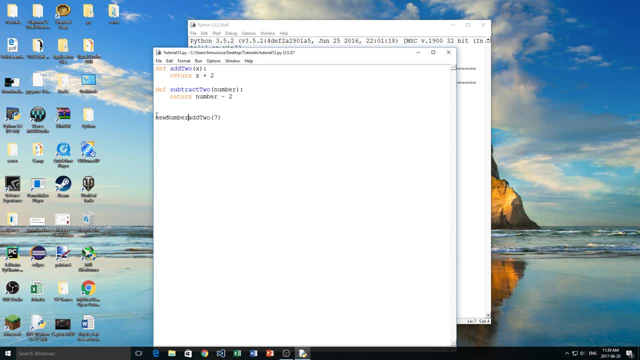 So I'll set it equal to a variable right now. so I'll say: newNumber is equal to addTo 7. And now, if I print out newNumber like this, we get 9.. Okay, so that's how that works. 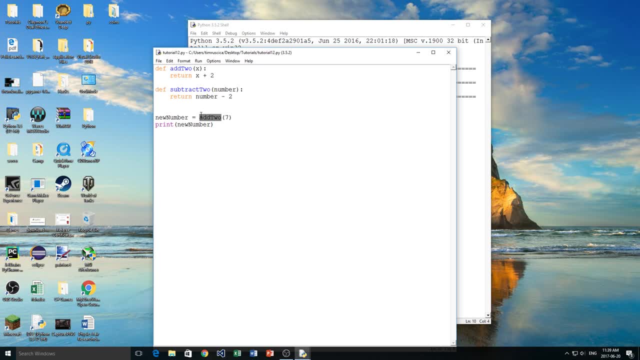 All right now what about subtractTo? So we can do the same thing here with 7, so we do subtractTo. We'll leave 7 in here for number and you'll see we get 5.. So that works correctly. 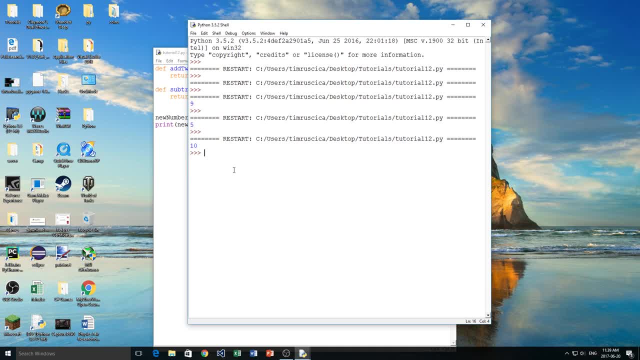 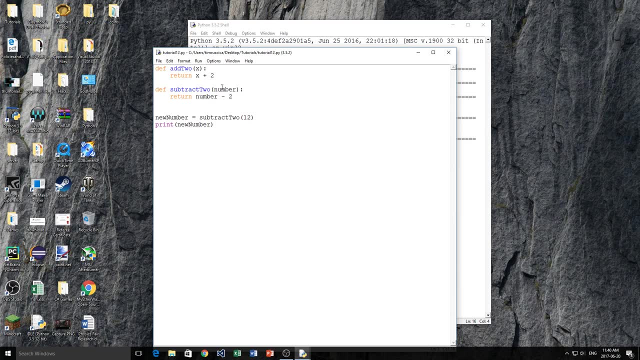 Now I can do it again. I can do 12, and we get 10.. And maybe I could even change what I want to do in these functions. So this one's called addTo, but maybe I wanted to add 2 to x. 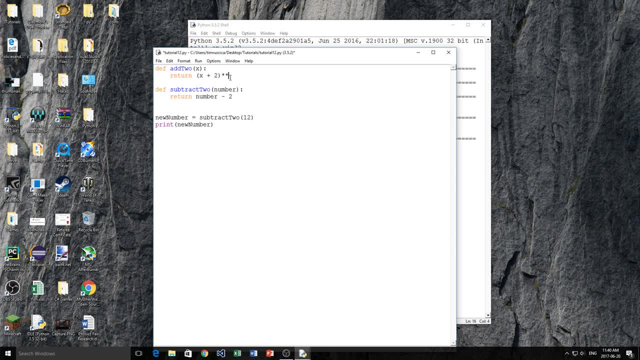 and then I wanted to square it, So then I would do that, and then, if we go back to the addTo, so I'm going to put 12 plus 2 squared, which would be 14 squared, which would be a pretty big number, which would give us 196, just like that. 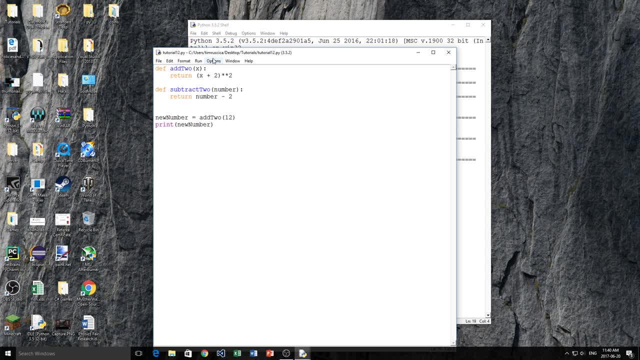 So you can kind of see and understand how these functions are working. They have a parameter. this is what that's called up here, So a variable name. I could do x, I could do y, I could do z, it doesn't matter. 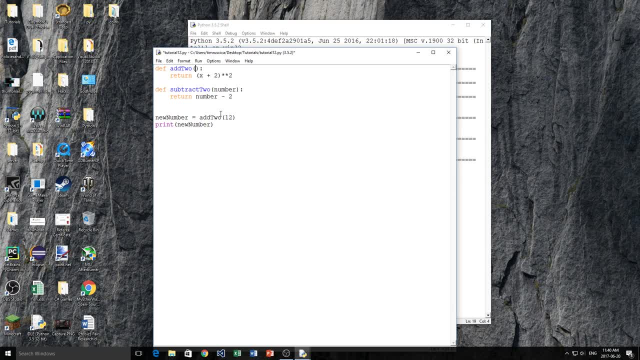 I can do any letter, I want any name, I want It makes sense to call it something That makes sense in terms of the function. So here x works fine, but if I was doing a string, so maybe we want to write another function. 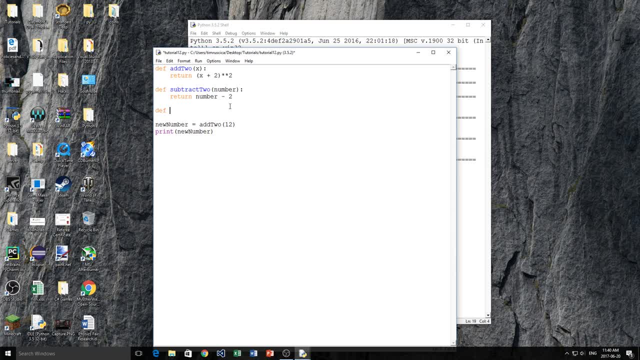 Let's do another function here and we'll do define and we'll say printString. And now inside of here, I'm just going to put string like that as our parameter name and then we're simply just going to print the string to the screen. 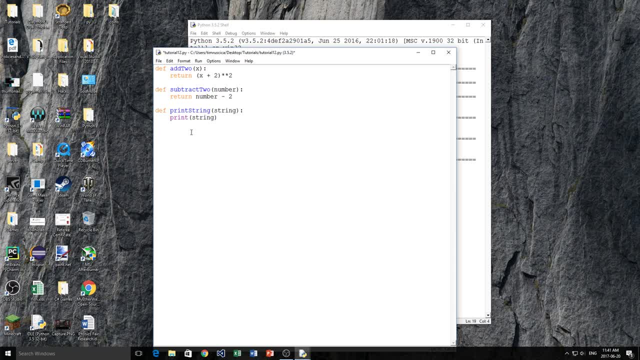 So now what actually happens is, instead of setting something equal to to a variable, all I have to do is I have to do printString- this is my call statement- and then in here I'm going to give it a string. So I'm just going to type hello, and you'll see if we run the function. 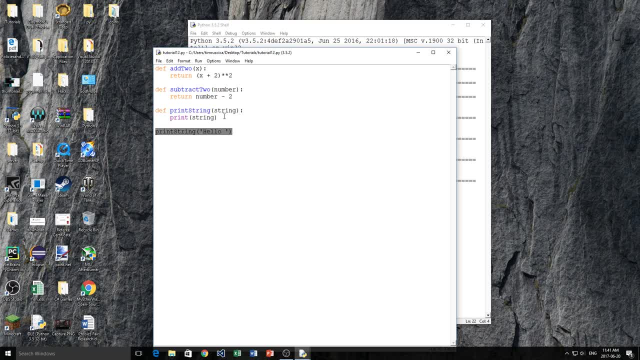 We get hello and we didn't print it down here, we just printed it from the function. So I know I've gone kind of fast, but the easiest way to understand the functions are to show examples of them and how they're working. 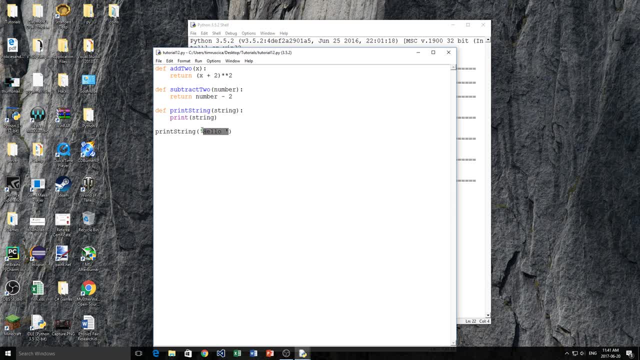 Pretty much. there's a parameter. I'm going to give the parameter. I'm in the argument of the call statement. So this in the definition of the function is called a parameter and in the call statement, in between the brackets, it's called an argument. 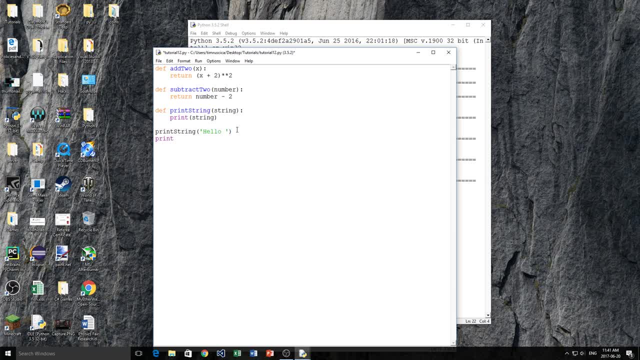 So those are just some key words. Now I can actually use these functions as many times as I want, So I can printString again and I can print: my name is Tim, just like that, and you'll see it should do it twice. yeah, there we go. 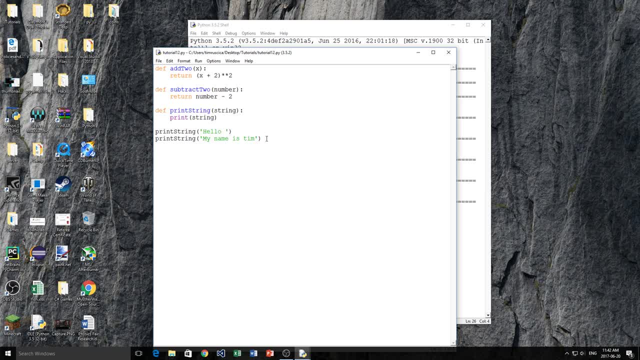 So that's why these functions are extremely useful, because, say, for example, I'm writing a big program and I know that I would need to do a certain thing multiple times. Well, I don't want to have to constantly write it out in the main line of my program here. 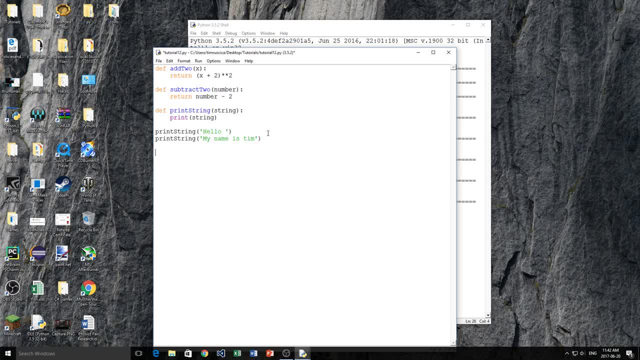 when I can just have a function that's going to do it for me and all I have to do is call that function using a simple call statement like this. So we haven't really done many big programs yet where functions make sense, but you'll see when you start programming that you're going to be using a lot of functions. 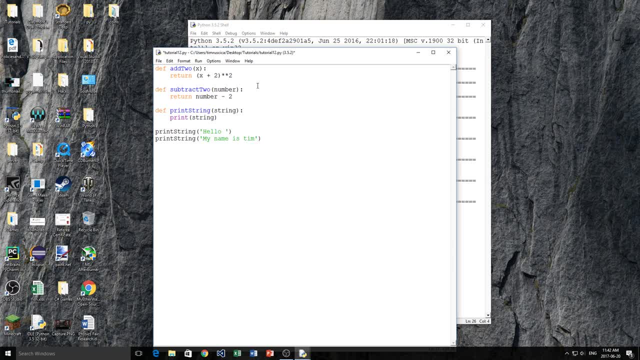 to do things because you're going to be repeating code. Now, these are very basic functions. We have subtract to add to, but you can have like physics functions. for example, If I know, I need to find the acceleration of an object. 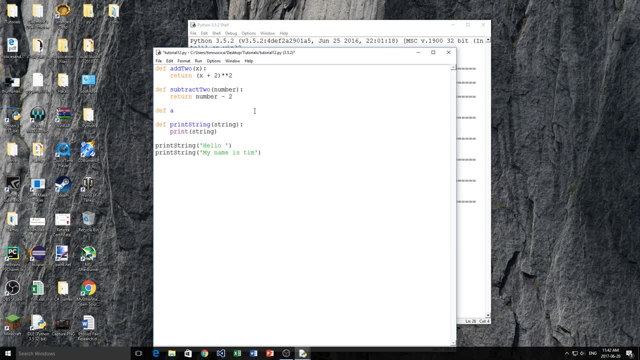 then maybe I would make another function here, and I do define Excel. I'll just do it like that short form and then I'll put in mass and the force, like that. So you see, I can actually have more than one parameter. 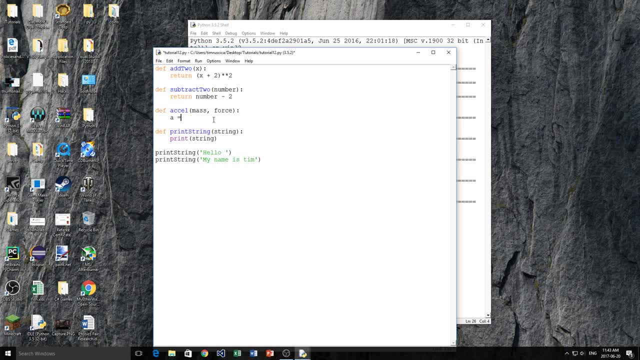 I can have two parameters here, and I'm going to say a is equal to mass times force. I know that's not correct, but we could do something like that- mass times force. And then I could return the variable a. And now if I called my Excel function and I printed that to the screen, 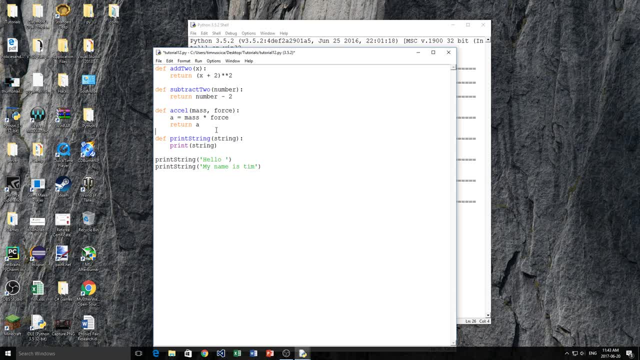 well, that would give me what the acceleration would be right. So those are just some examples of why functions are extremely useful. We're going to talk more about functions. I'll do a more advanced tutorial a little later on, but this is just an introduction. 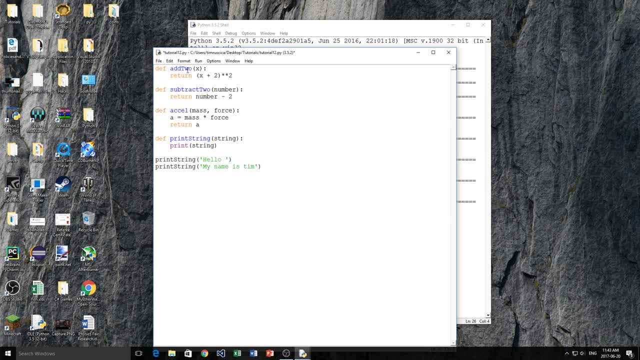 so that you can have a little bit of fun. Hopefully you understand how they work. Pretty much you have. if you're writing a function, you have the def keyword, You have the function name, so in this case it's highlighted in blue. so I did add to.